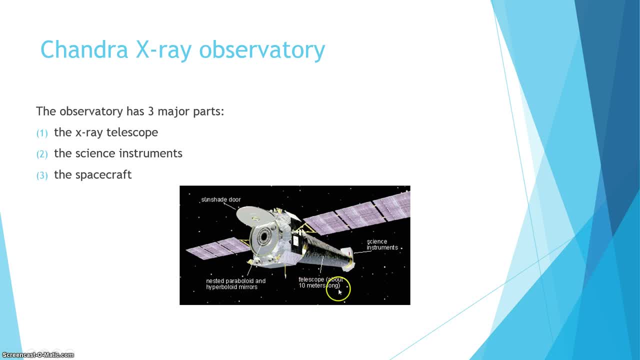 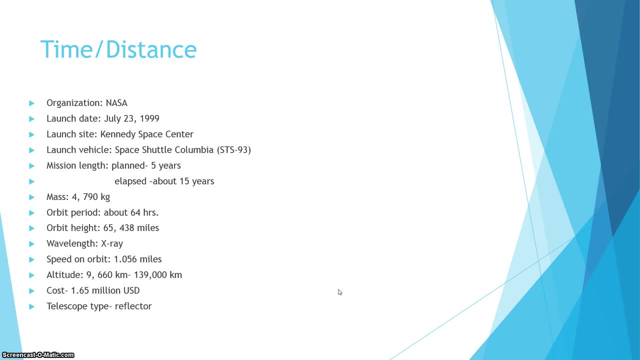 and around here is the telescope, which is about 10 meters long. Chandra was launched on July 23, 1999, from the Kennedy Space Center, Florida. The vehicle was a Spatial Columbia. Chandra was the first spacecraft to be launched in the United States. 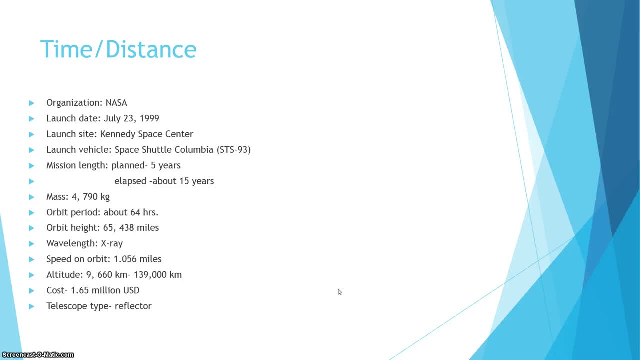 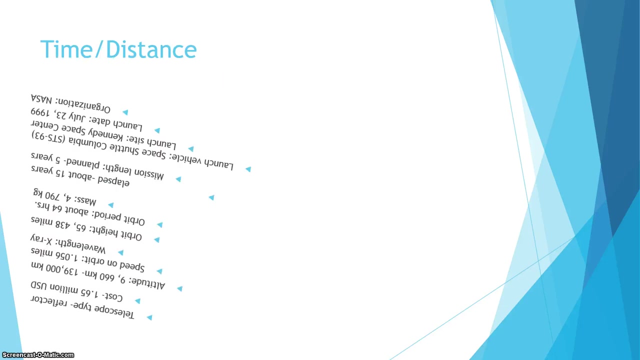 The mission was originally planned for 5 years, but was extended to about 15 years due to the usability it provided. The height of Chandra's orbit was 65,438 miles and the orbit period was about 64 hours. Chandra's Purpose. 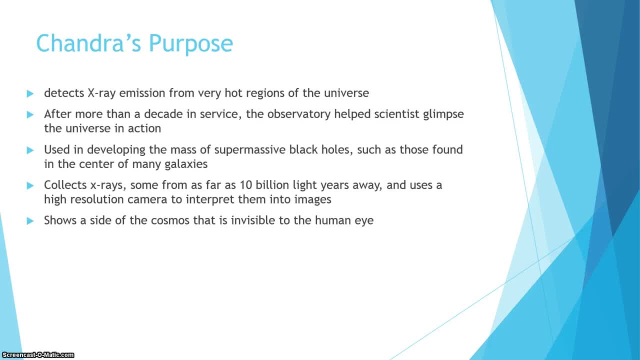 The telescope was specially designed to detect X-ray emissions from very hot regions of the universe, such as exploding stars, clusters of galaxies and matter around black holes. After more than a decade in service, the observatory helped scientists glimpse the universe in action. watch galaxies collide. 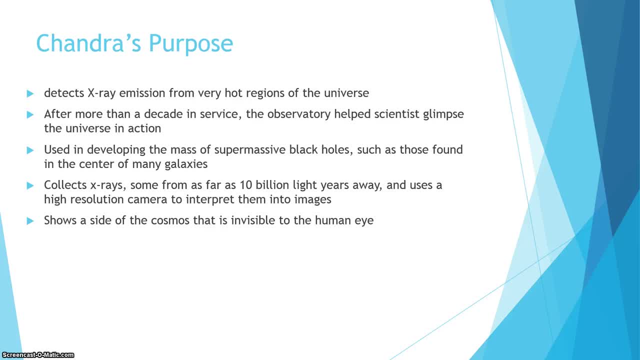 observe the black hole with cosmic hurricanes, and watch a supernova turning itself inside out after an explosion. Chandra collects X-rays, some from as far as 10 billion light-years away, and uses a high-resolution X-ray system to detect X-ray emissions from very hot regions of the. 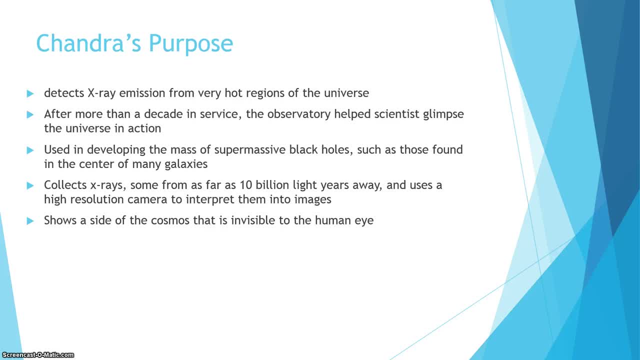 universe. Chandra has a high-resolution camera to interpret them into images. Also, Chandra shows a side of the cosmos that is invisible to the human eye. To summarize everything that I've said so far, Chandra is a sophisticated, state-of-the-art instrument that represents a tremendous technological advance in X-ray. 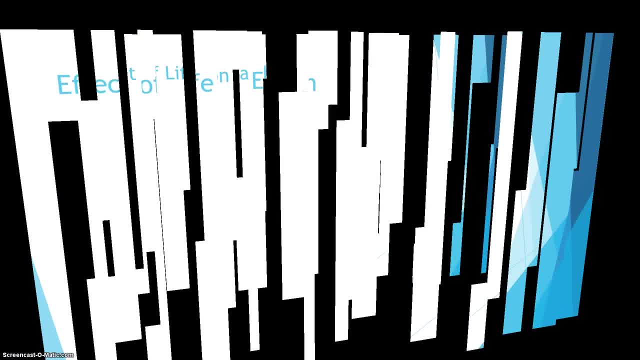 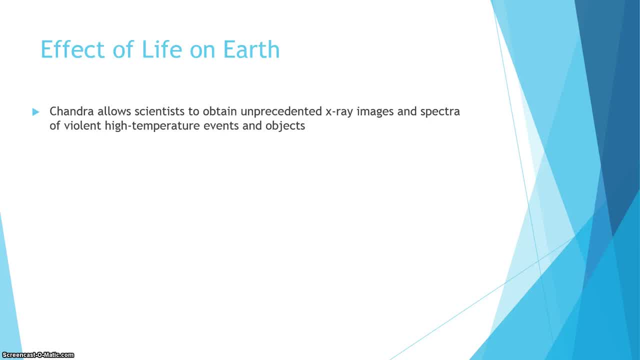 astronomy Effect of Life on Earth. Chandra allows scientists around the world to help them better understand destruction and evolution of her universe. They have used Chandra to learn more about the dark matter that may make up most of the mass of the universe. study black holes in detail. witness the results of supernova explosions. 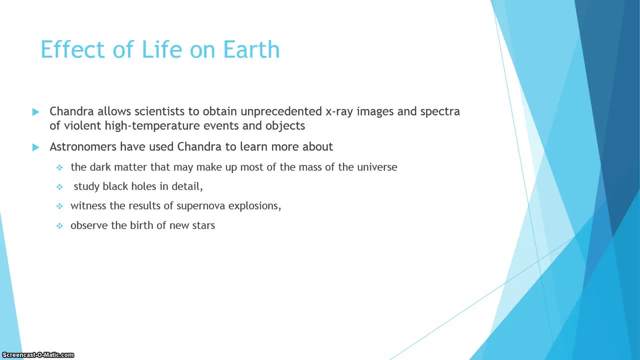 and observe the birth of new stars. It gave astronomers a new tool for determining if a planet-forming disk surrounds a young star. Using Chandra, astronomers have found that the growth of galaxies containing supermassive black holes can be slowed down by a phenomenon.